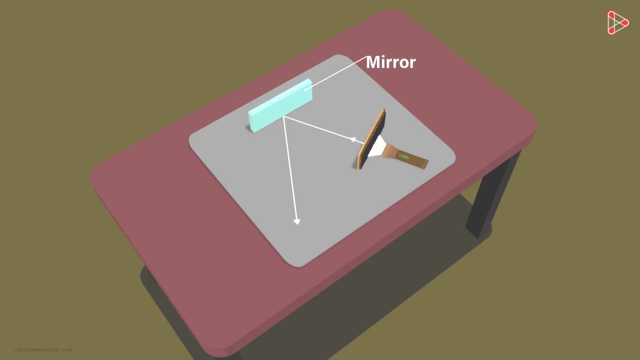 Next, we place the plane surface of the mirror in the path of this light. What did you see? Did the light get reflected? Yes, you can clearly see the reflection of light on this sheet of paper. Represent this light with the incident ray and reflected ray. 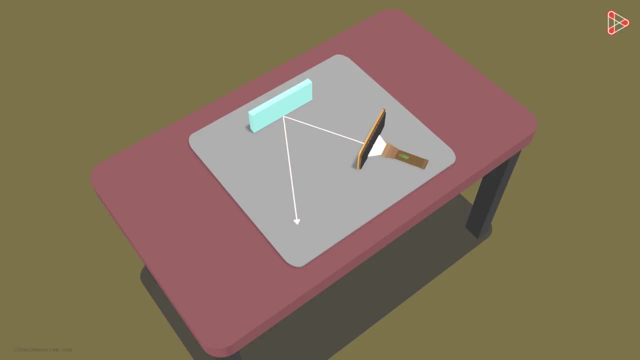 drawn on this white sheet of paper like this. Also draw a normal to the mirror surface. Remember, normal is a perpendicular line drawn at the point of incidence. What are these two angles called? This angle is called angle of incidence and represented by I. 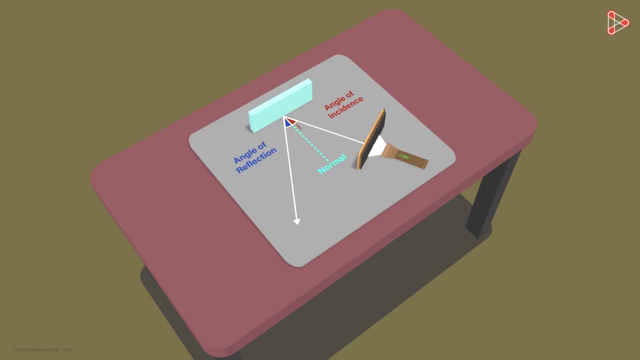 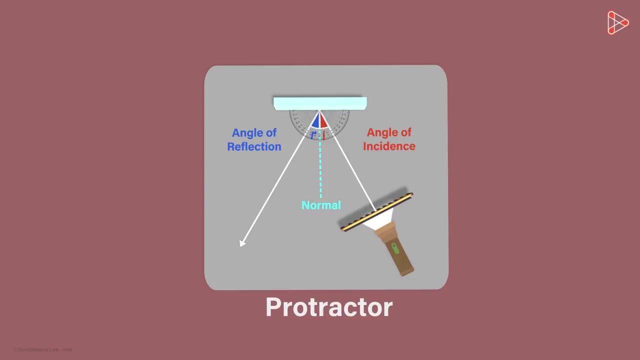 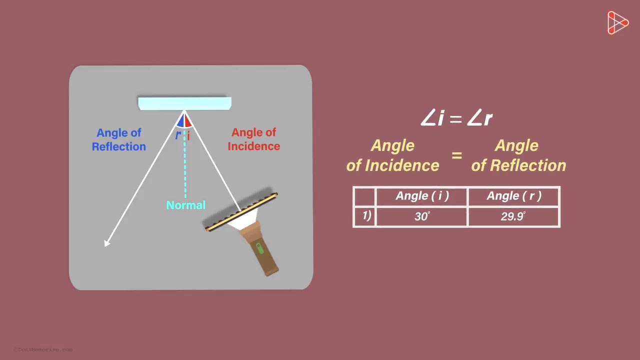 while this angle is called angle of reflection, represented by R. Measure these two angles with the help of a protractor. The measure of the two angles will almost be the same. They are approximately equal. This is the first law of reflection, So with this experiment you can verify this law. 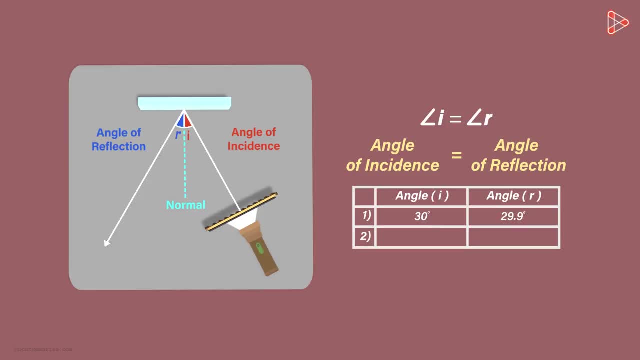 Well, if you are still not convinced, you can take further readings by changing the direction of the incident light. Change this angle of incidence by moving the comb slightly. Make sure that the point of incidence is the same in both cases, That is, this point here is same as it was previously. 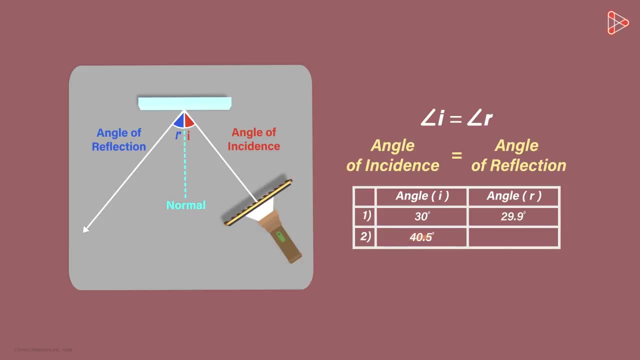 But notice that this time the angle of incidence is greater than the previous one. So by the first law of reflection of light, the angle of reflection should also be greater, And that is the case, indeed. Measure both the angles and again you will find that they are approximately equal. 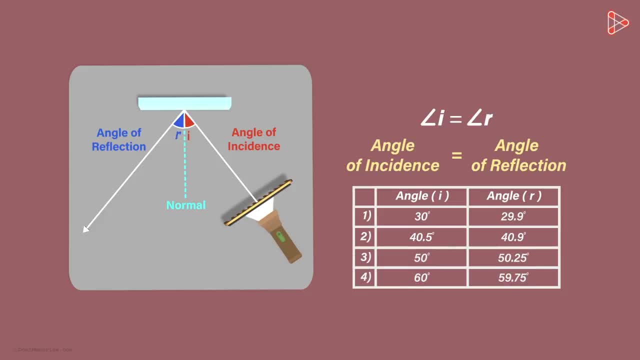 Take two more readings to complete this table. Do you notice anything strange here? The first law tells us that angle of incidence is equal to the angle of light. The second law tells us that angle of incidence is equal to angle of reflection and not approximately equal. 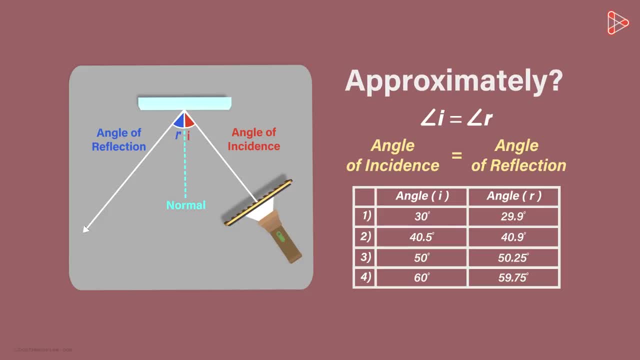 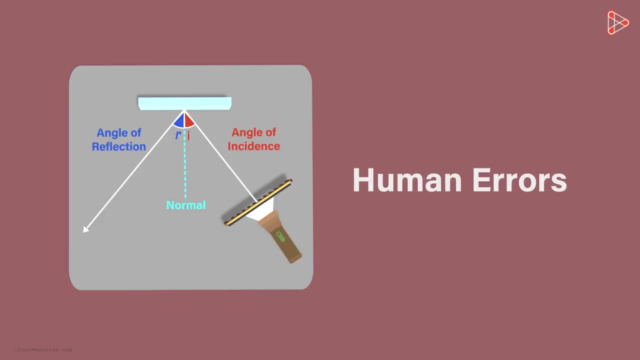 Why am I using the word approximately? Well, there are chances of errors that may come about during measurements of things. We can refer to them as human errors. It also depends on narrowness of the light beam. Narrower this beam, more accurate will be the results.